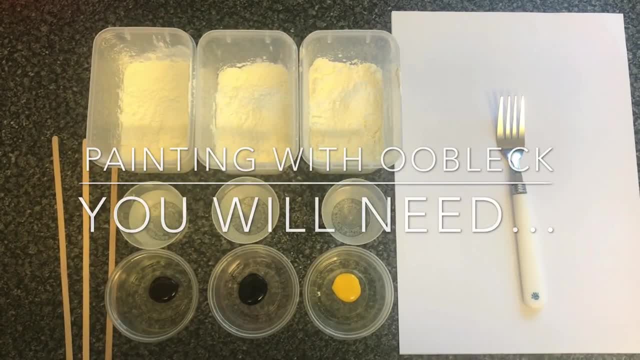 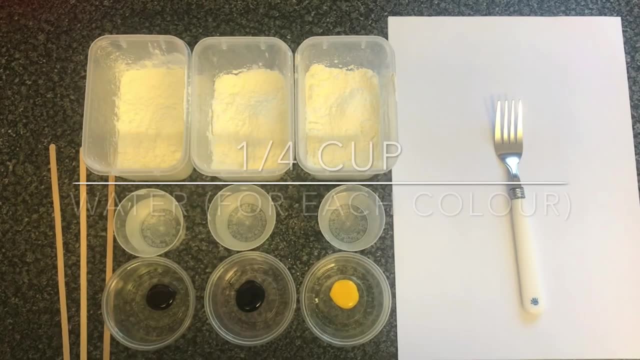 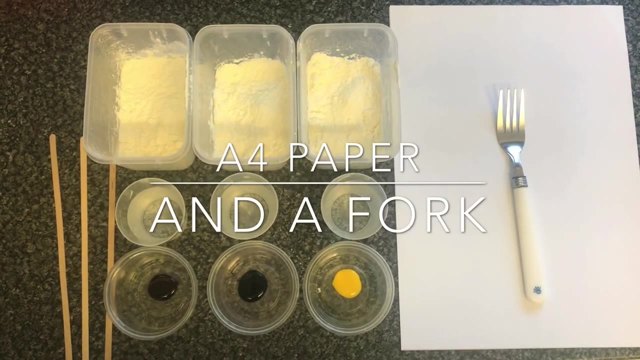 For the painting with oobleck activity, you will need half a cup of cornflour for each colour that you are going to use, a quarter cup of water and food colouring. You will then need a piece of paper and a fork for the painting. 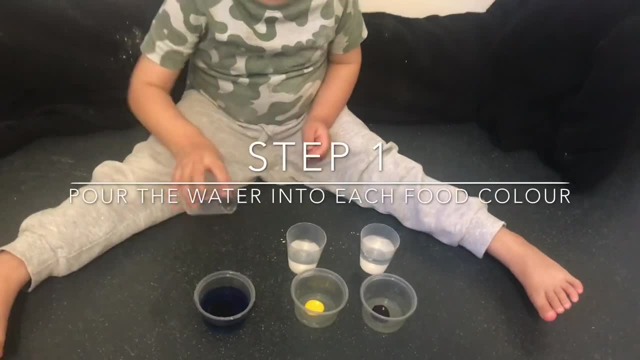 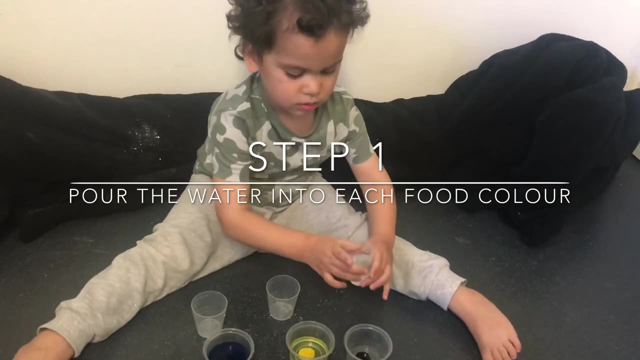 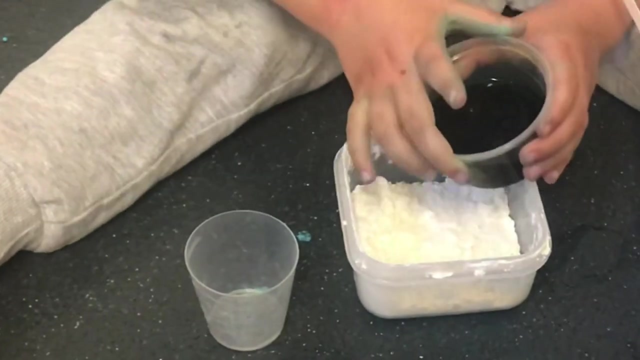 The first thing we're going to do is place the water into each of the different food colouring, Then we're going to give it a mix and then pour the coloured water into the cork. Mix it up, Mix it up. Now it's time to paint with the oobleck. 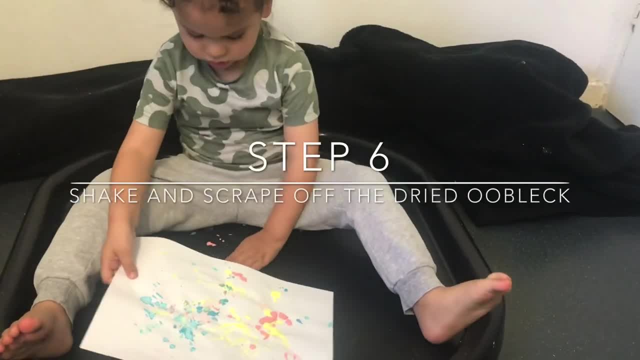 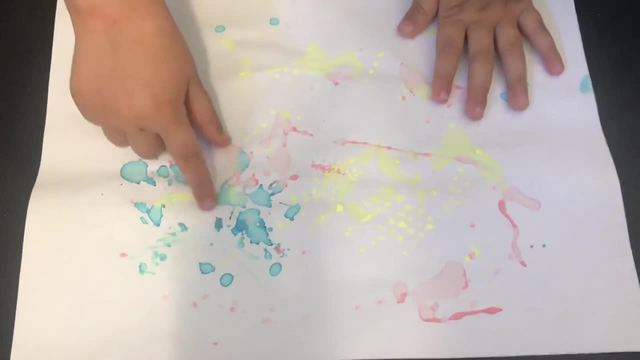 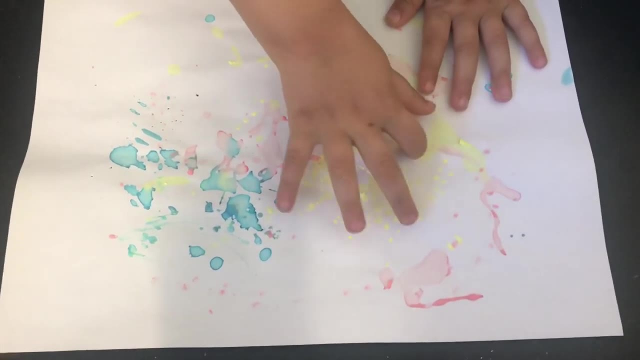 Allow it to dry. Once dry, it's time to shake off all of the dried oobleck. If there are any dry bits left behind, just scrape it off and there you have your beautiful oobleck painting. Activity five is colour mixing with the oobleck. 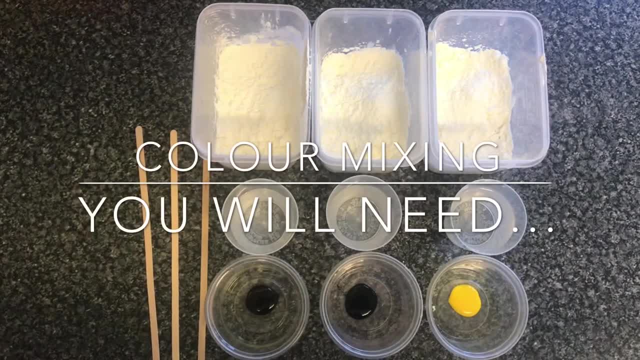 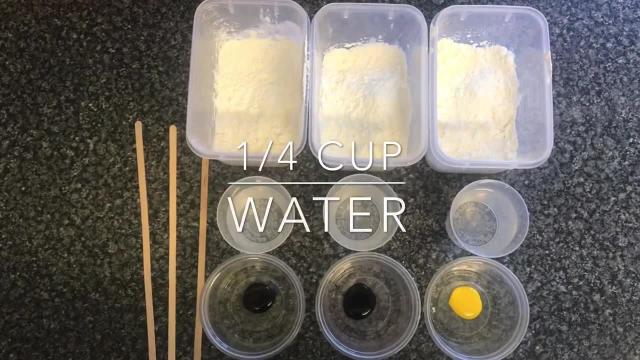 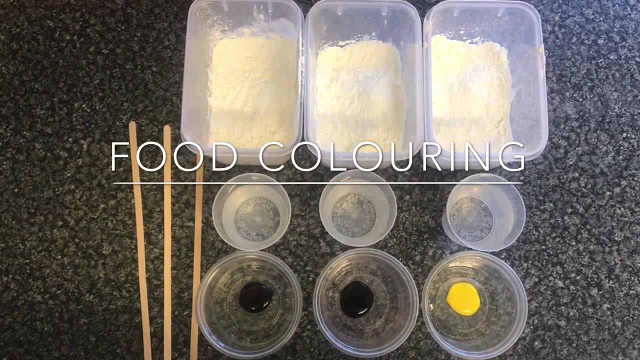 For the colour mixing activity you will need. for each colour you are using half a cup of cornflour, a quarter cup of water and food colouring. So we're using the primary colours- red, blue and yellow- and we are going to colour mix the oobleck. 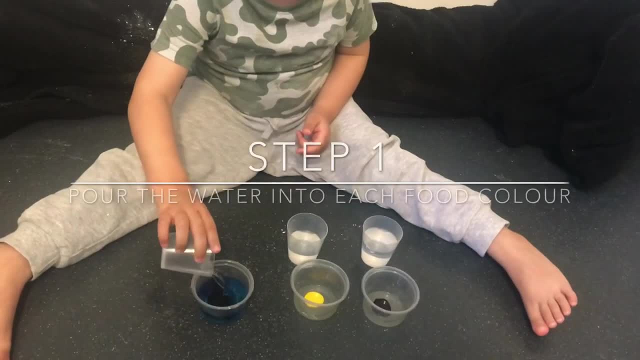 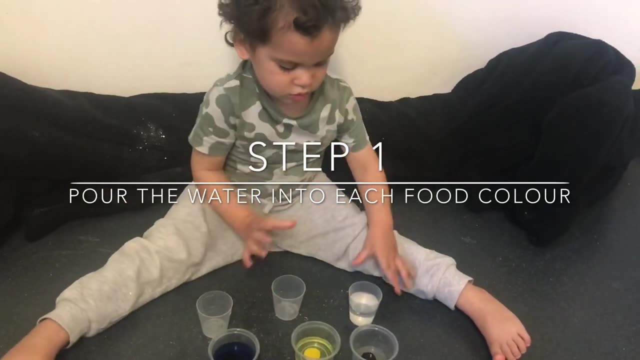 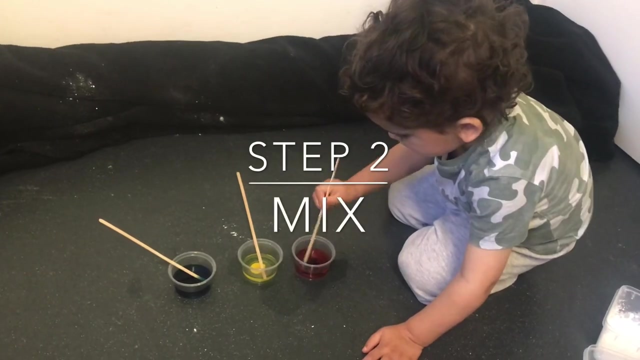 to make our secondary colours. So the first thing we're going to do is place the water into each of the different food colouring, Then we're going to give it a mix and then pour the coloured water into the cornflour, Then mix it up. 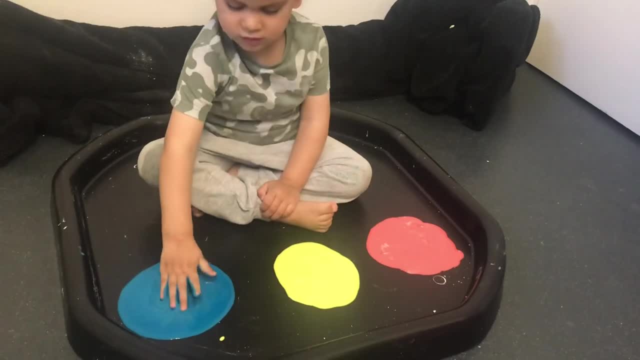 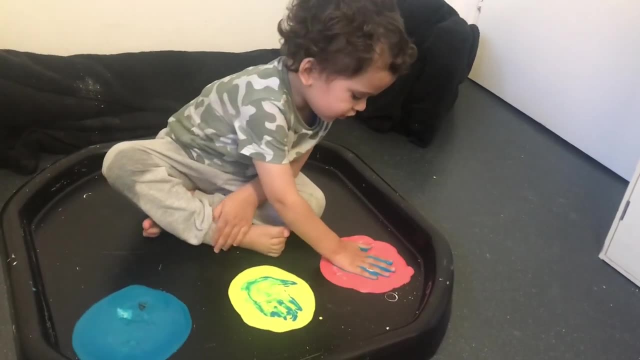 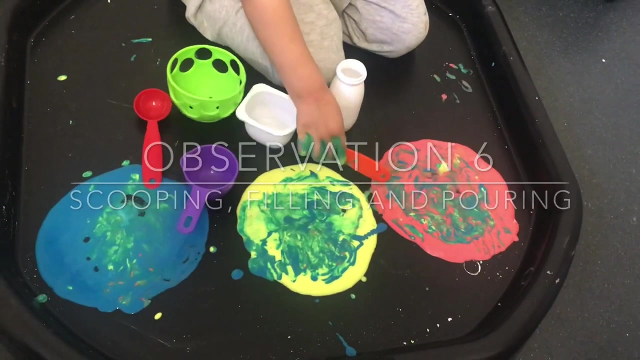 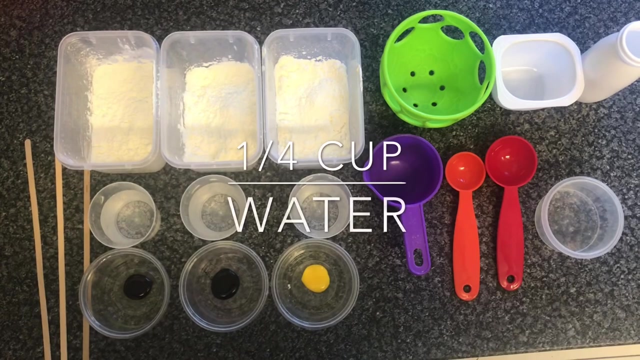 Mix it up, Look Ta-da. Activity six is scooping, pouring and filling with the oobleck. So for this you will need half a cup of cornflour, quarter cup of water and food colouring, And then containers and spoons.